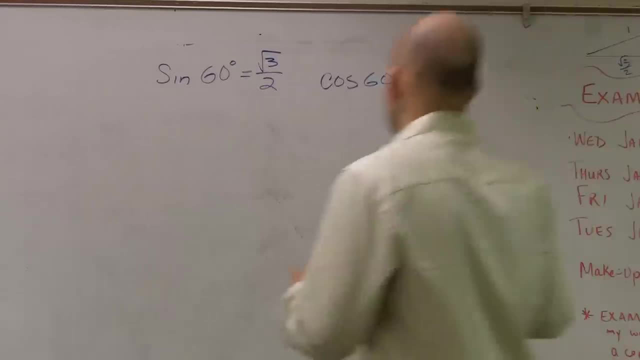 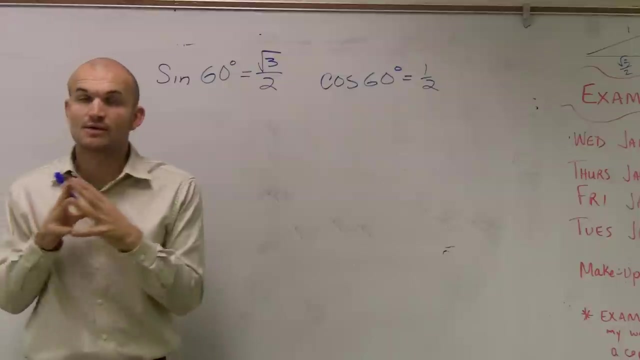 All right. So what we have is we have two angles. We have sine of 60 degrees equals square root of 3 over 2, and cosine of 60 degrees equals 1- half. Now there's a couple things I want you guys to remember that we're going to have to use for this. 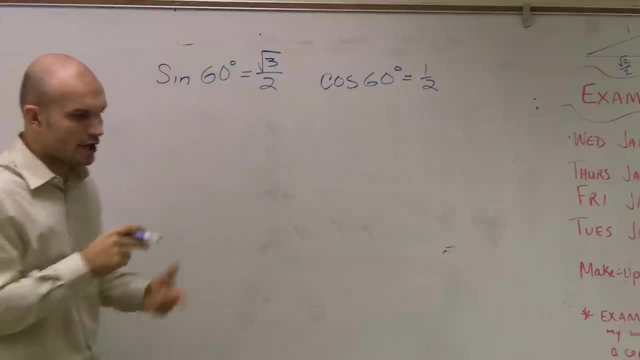 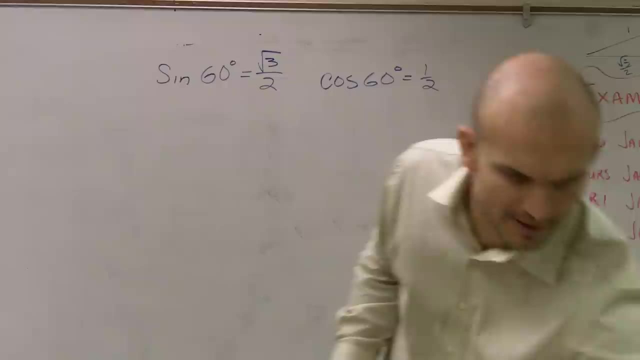 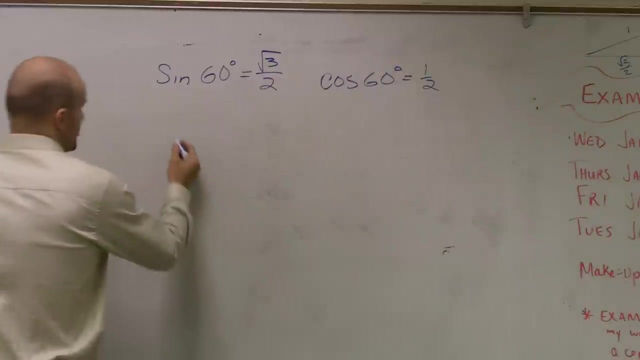 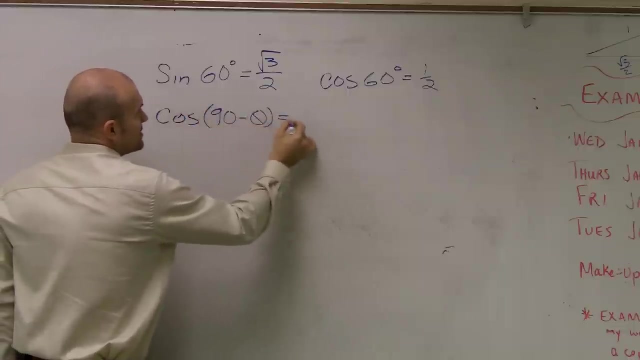 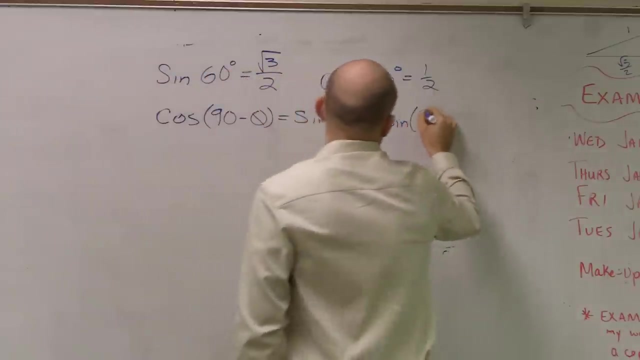 First of all, we need to know our trig properties And we also need to know what our co-functions of complementary angles. So what I'm saying is we need to understand that cosine of 90 minus theta is equal to sine of theta, And we also need to know that sine of 90 minus theta. 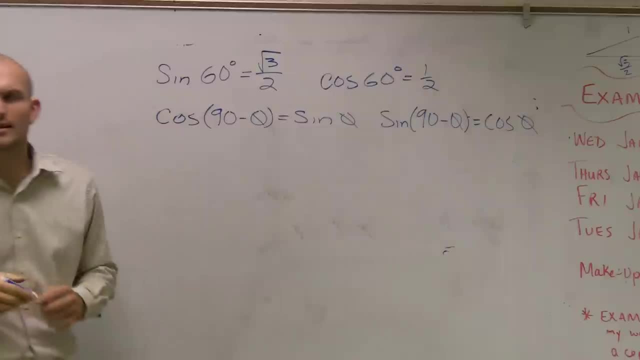 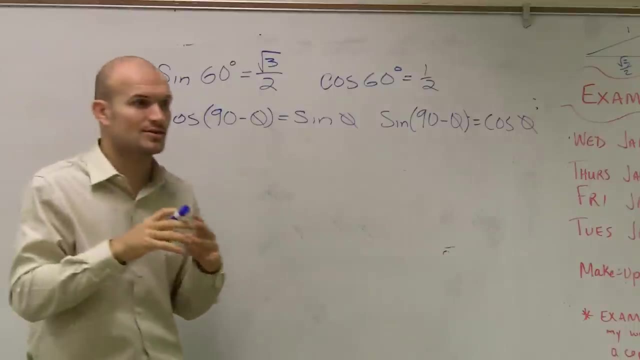 is equal to cosine of theta. This was actually below your blue box. I'd recommend that you guys write these down if you didn't have them. If you look at that blue box- on page 282, we have these written down. I told you guys to write down the blue box. 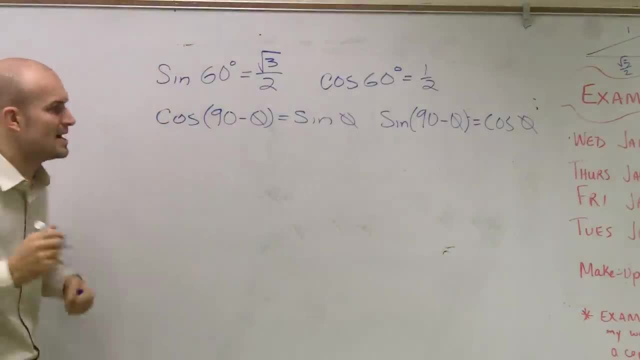 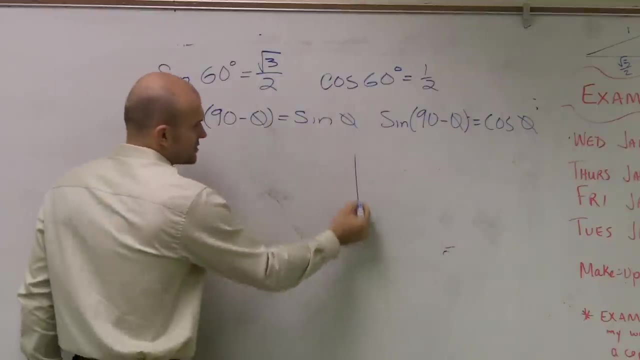 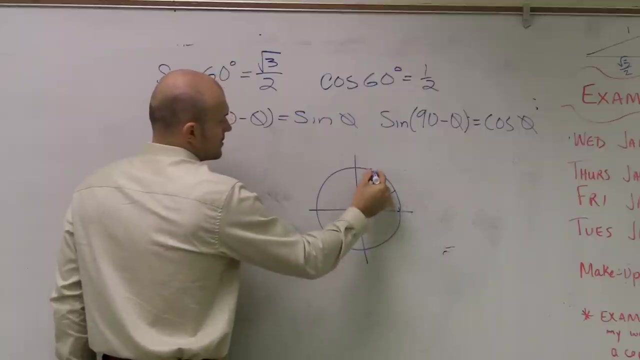 I didn't mention these, But if you guys don't have these written down, I'd recommend you write them down. I did go over last class period. why this works, If you remember, you look at a unit circle And let's see. 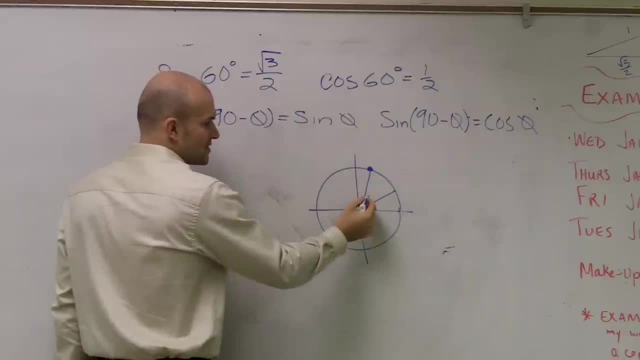 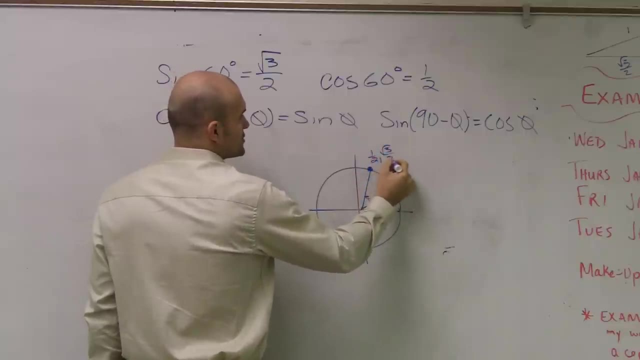 This one is what we say for cosine: That's 60 degrees, right, And that's 30 degrees. So, if you guys remember, this point was 1 half radical, 3 over 2.. This point is radical 3 over 2 comma, 1 half. 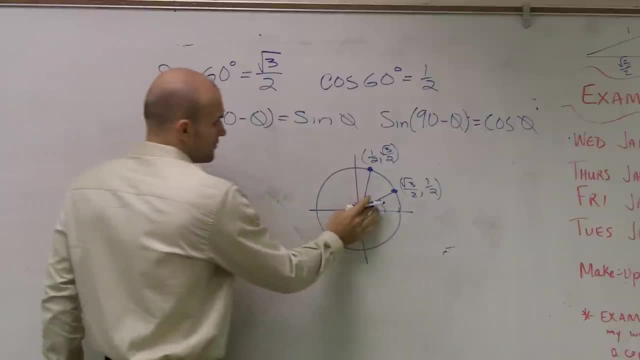 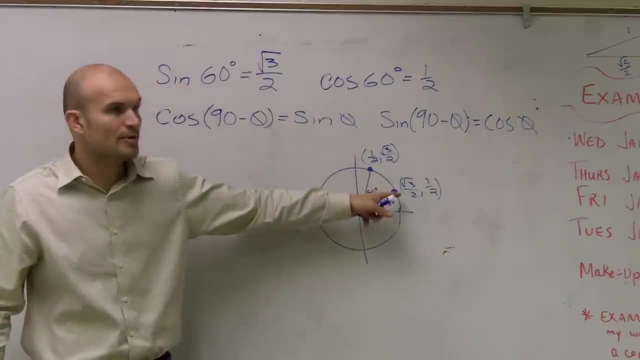 On your unit circle, you guys remember those. Well, this angle, remember, is 60 degrees And this angle is 30 degrees. in degree form, We said this is pi over 6, and that's pi over 3.. But 30 degrees and 60 degrees, 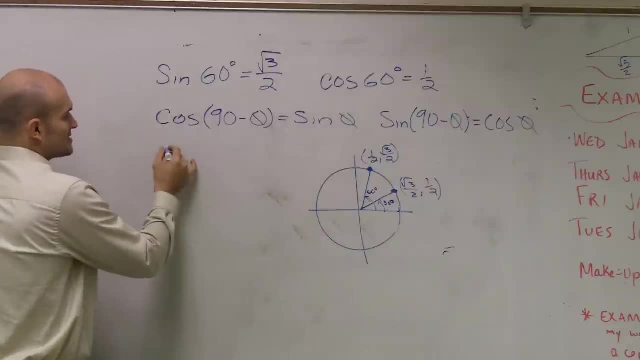 Well, look at it. If I say, what is, I don't know, The cosine of 60 degrees is 1 half, So the cosine of 90 minus 60 degrees is the same thing as well. if cosine of 60 degrees, 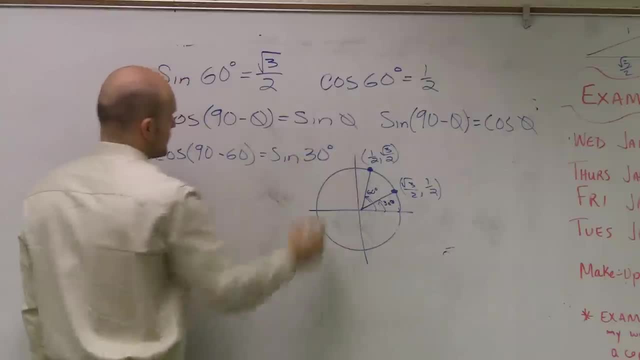 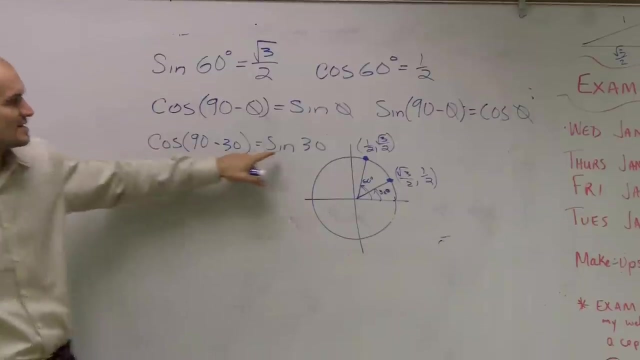 is actually going to be the same as sine of 30 degrees. I'm sorry, 90 minus 60. Is cosine of 60, right, Is 90 minus 30 is 60? So the cosine of 60 degrees is the same thing. 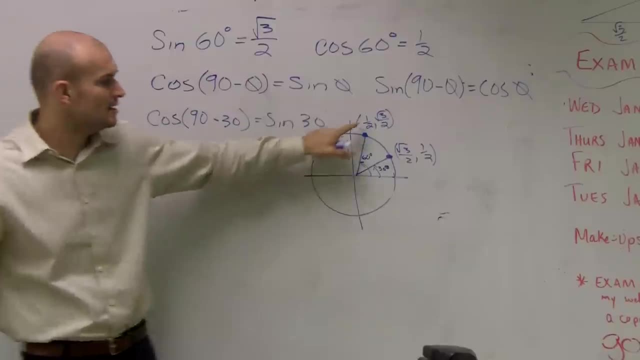 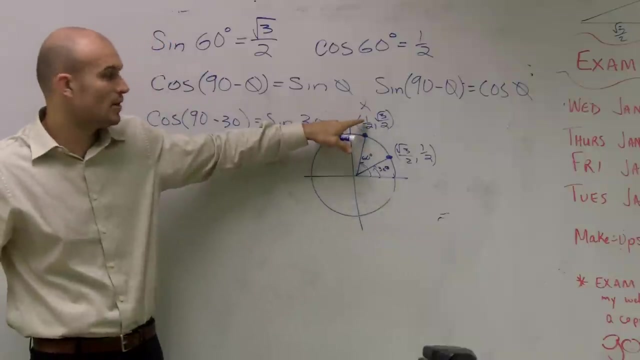 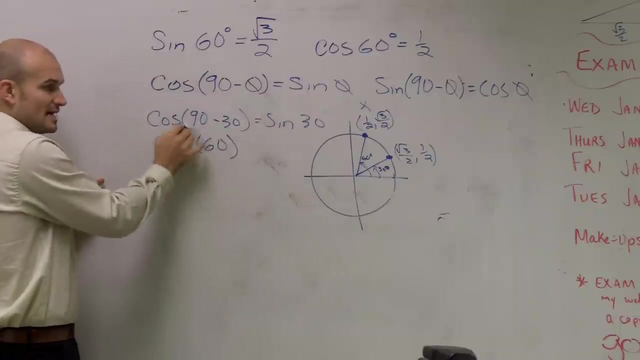 as the sine of 30.. Let's see if that works. What is the cosine of 60 degrees Cosine? is your x value right? The x value of this point is 1 half And I said the cosine 90 minus 30 is 60.. 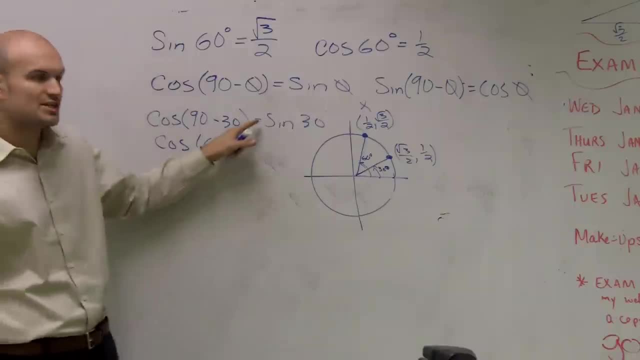 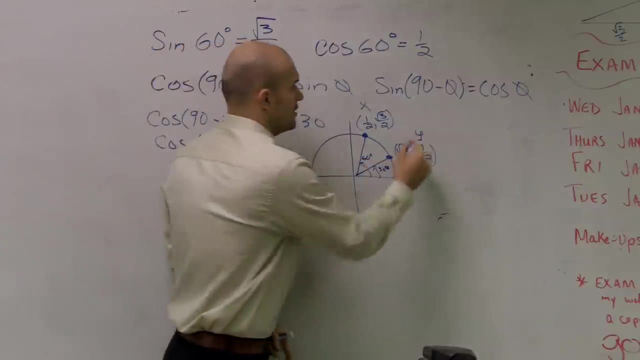 That's the same thing as cosine of 60 degrees. Cosine of 60, we just said, is the same as sine of 30. What is the sine of 30 degrees 1 half? OK, Huh, I'm confused on why you're going. 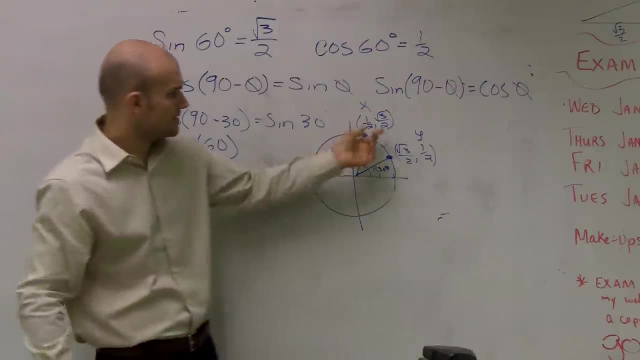 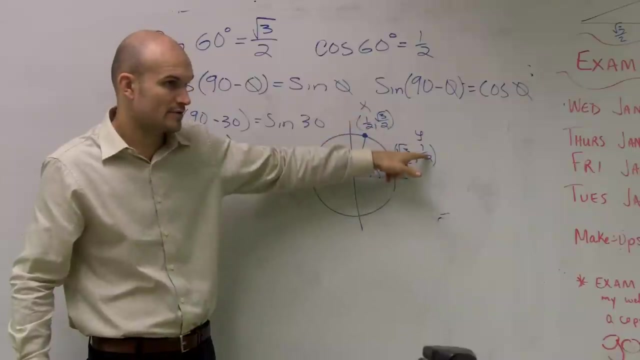 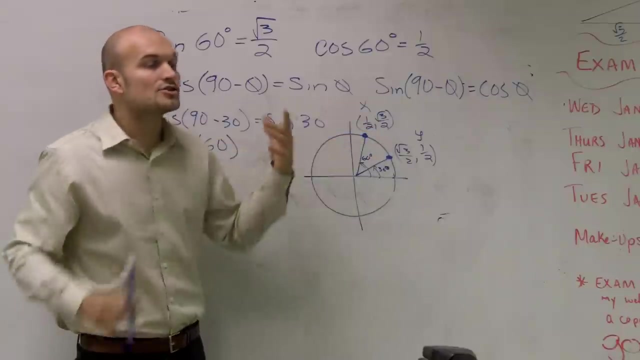 into sine of 30 degrees. What I'm saying is, if you look at this, the cosine of 60 degrees is equal to the sine of 30 degrees. Do you see how those are both 1 half Same thing? The cosine of 30 degrees is the same as the sine of 60 degrees. 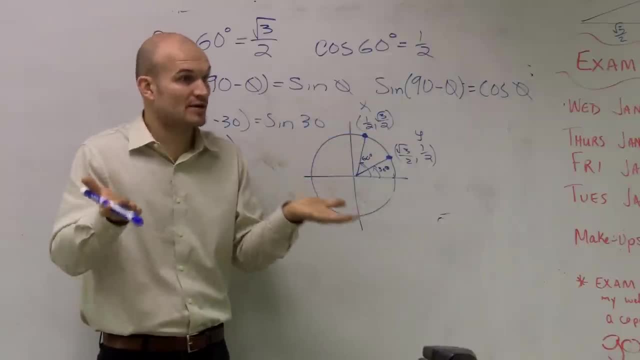 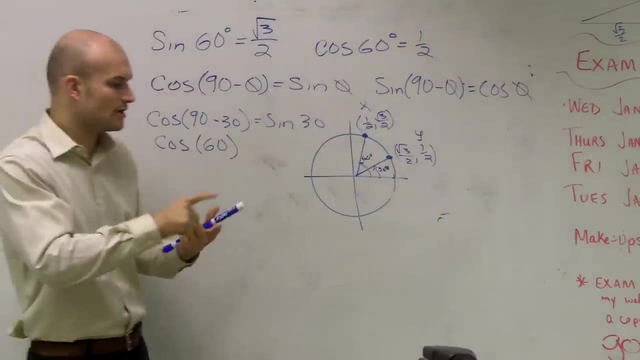 So think of 60 and 90.. 60 and 90. They're what we call complementary angles, Correct: 30 plus 60 equals 90 degrees. So what we're saying is these two functions, and it works for your secant and your cotangent as well. 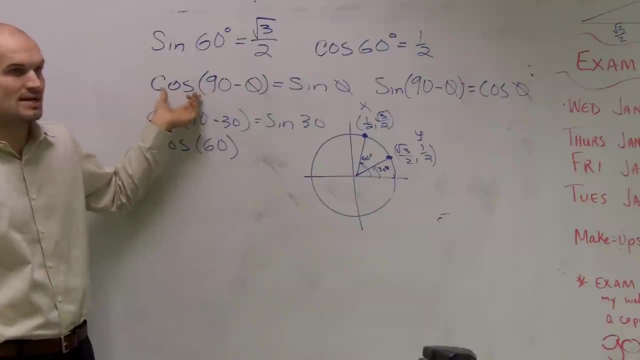 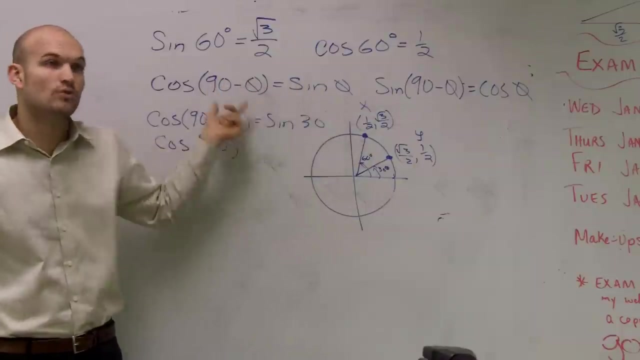 But what I'm saying is, if I know one angle in cosine and I subtract that from 90, what I subtract that from is going to give me my sine of that angle. They're equivalent, OK. So let's work out and see how this 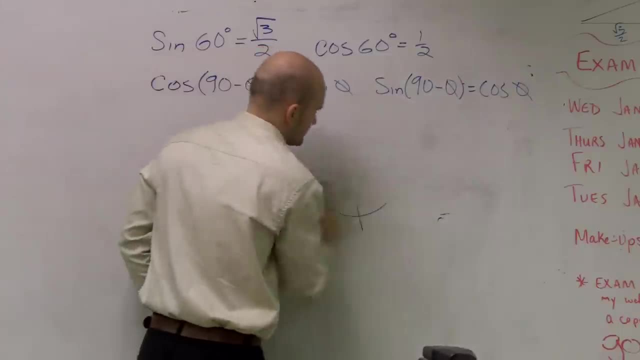 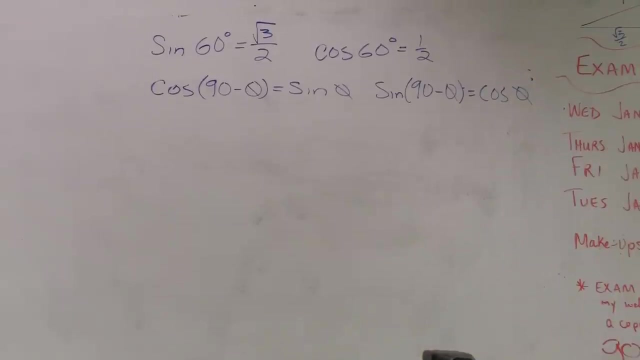 is going to work for our problem, Because what it asks us to do is for this problem. it actually asks us a couple questions They want us to find OK. So what they want us to do is they want us to find these angles. 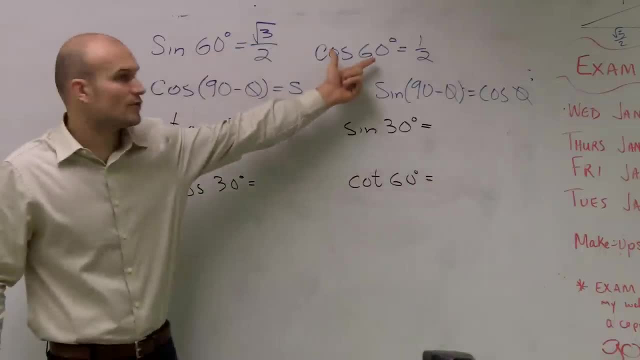 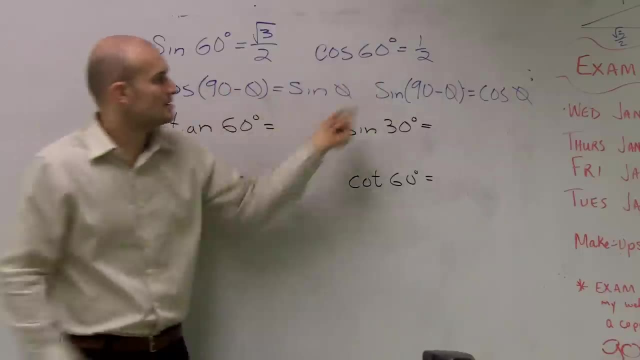 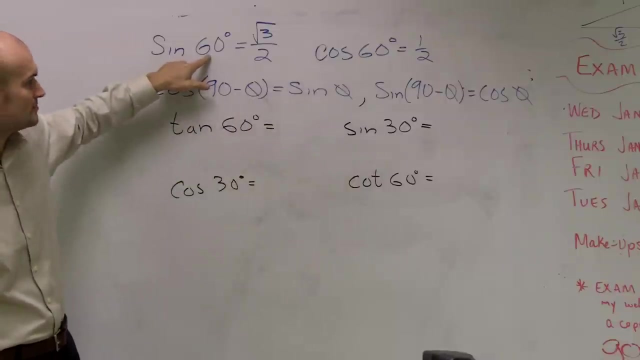 Well, let's think about it, guys. We only know what the 60 are for cosine and sine right. We only know what those are. However, we know by our co-functions, complementary, co-function identities, that what I can do is the sine of 60 degrees. 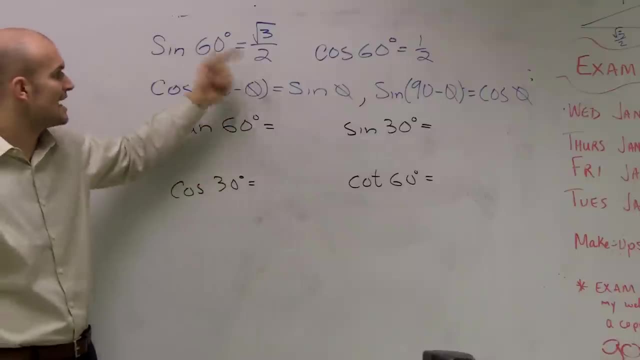 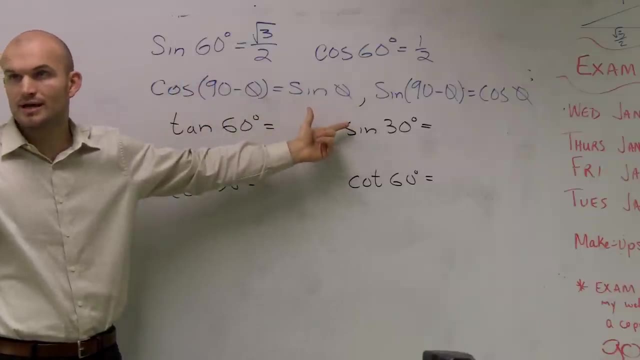 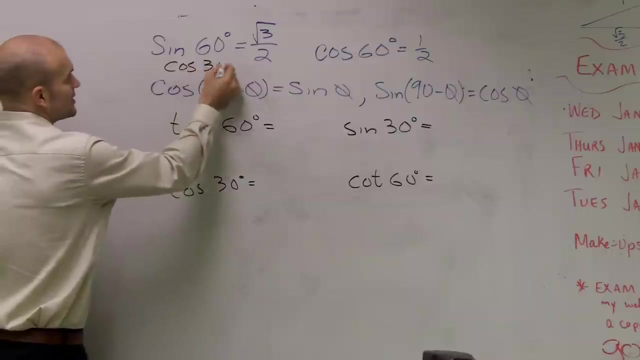 if I plug that in, the sine of 60 degrees is the same thing as the cosine of 30 degrees. by plugging it in by using these co-function identities- No, Did I get everybody with that? The sine of 60 degrees is equal to the cosine of 30 degrees. 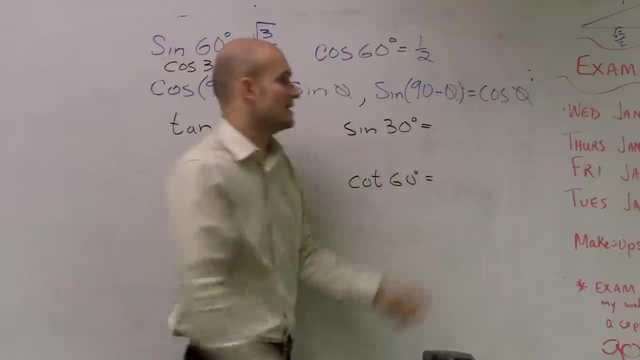 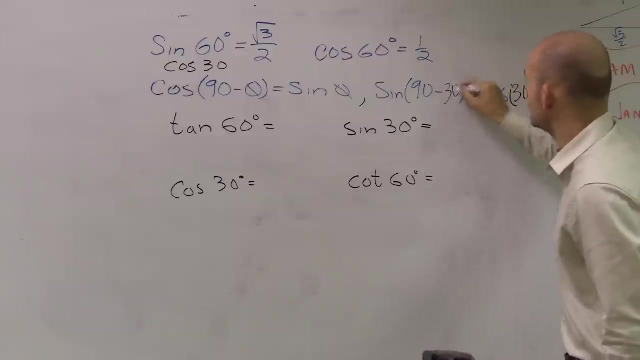 Let me go and show you. Let's look at it. If I replace theta for 30, and I place theta over here with 30,, 90 minus 30. OK, The sine of 30 is 60.. The sine of 60 degrees is equal to the cosine of 30 degrees. 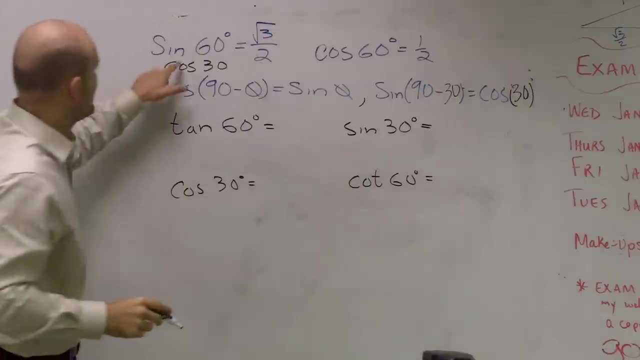 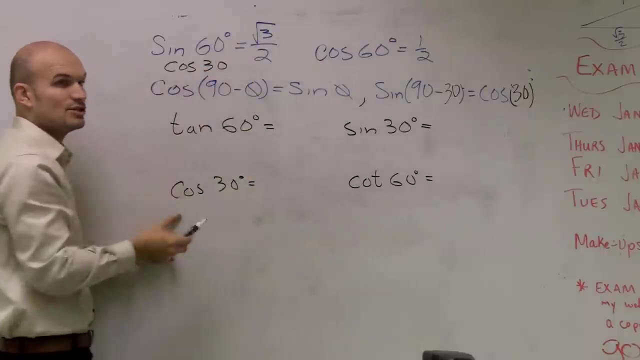 Does that make sense? OK, So therefore, if I say the sine of 60 degrees is pi over 3 over 2, and they tell me what is the cosine of 30,, I know that these two are equal to each other, right? 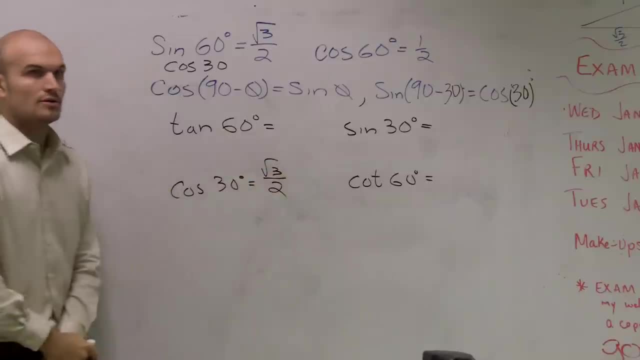 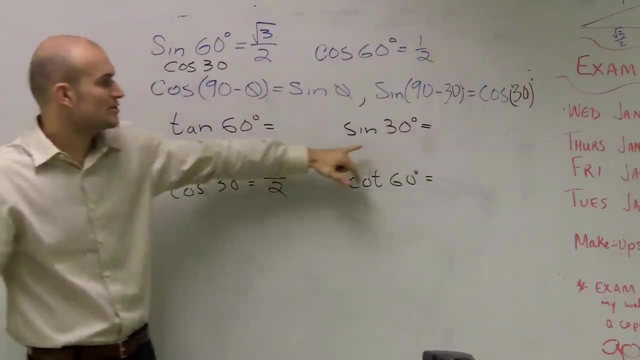 So this answer is very easy. The only thing you need to know is understand these complementary co-function identities. All right, Then let's look at the sine of 30 degrees, The sine of 30 degrees. let's put in 30 degrees for here. 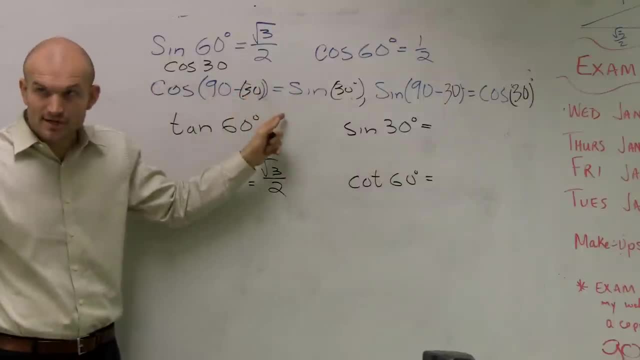 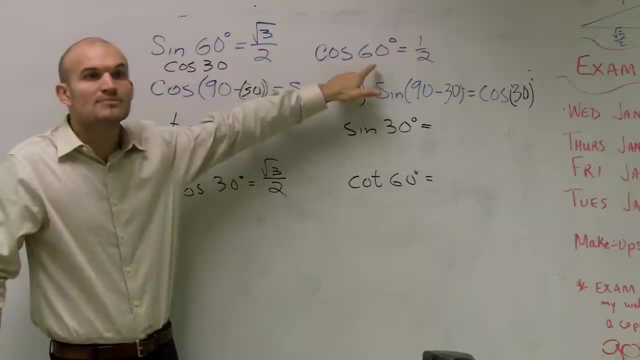 The sine of 30 degrees is the exact same thing as 90 minus 30,, which is 60. So the sine of 30 is the same thing as cosine of 60. Our original problem said cosine of 60 is 1 half. 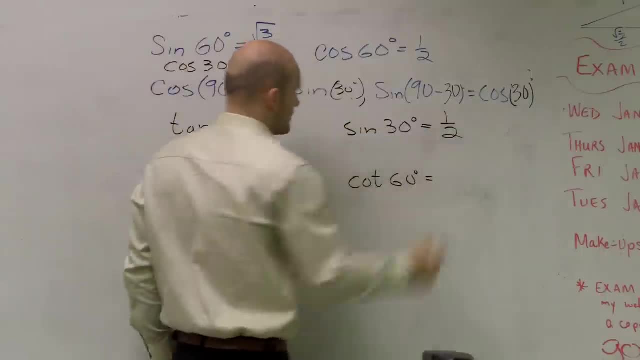 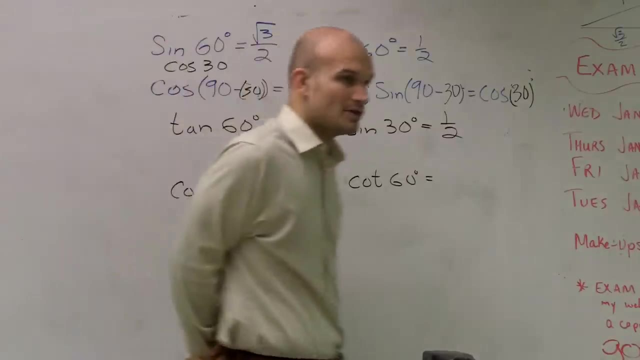 That make sense. OK, Now how do you figure out what tan of 60 is and what cotangent is? Well, we could actually create a right triangle and figure that out. That wouldn't be anything that would be difficult to do. 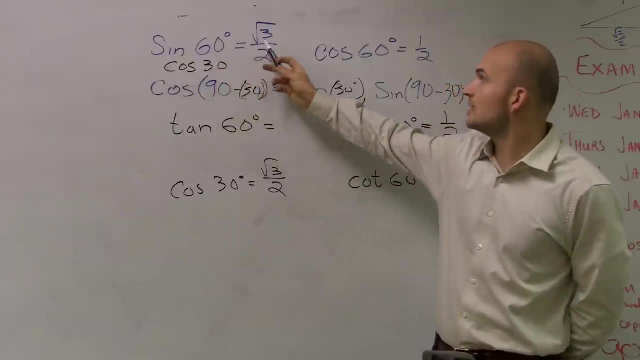 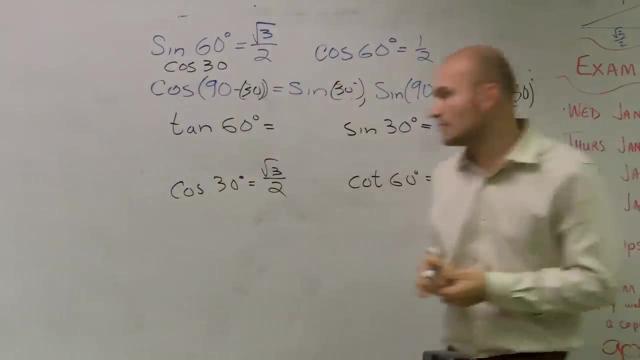 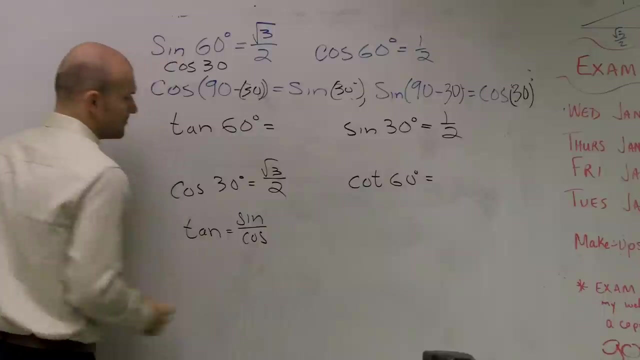 We could say: sine is a 60 degree angle, which is square root of 3 over 2.. You could create a triangle and figure out your tangent and your cotangent. However, another way you guys can look at this is: we also know that tangent is your sine over your cosine. 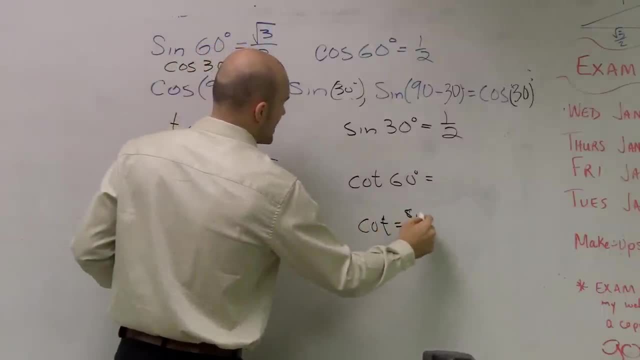 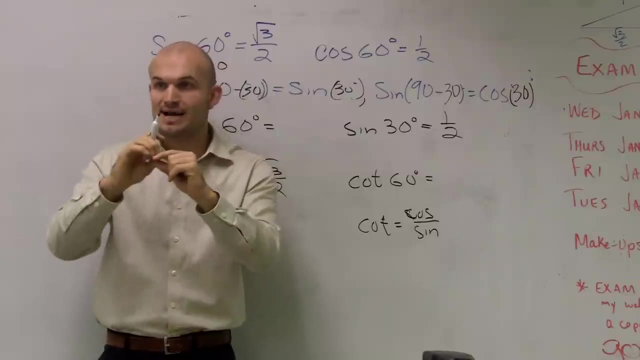 And cotangent is equal to your cosine. Cosine over your sine right. Remember when you guys were finding coordinate points We said, like the x and the y or the y and the x, right? Well, y represents your sine and your x.